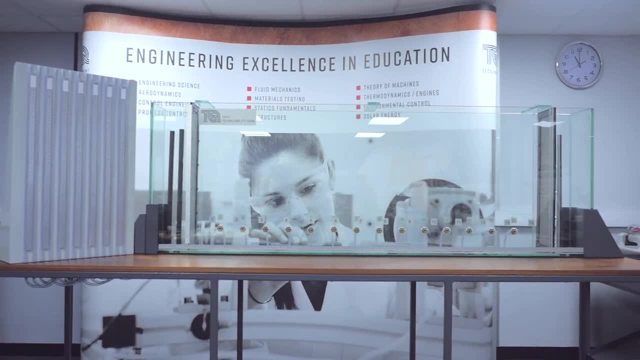 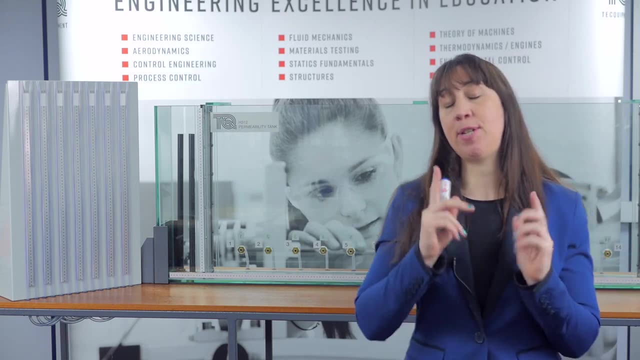 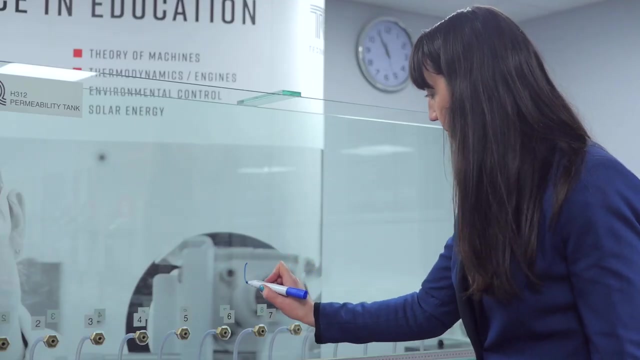 upstream and downstream sides of the dam. With a concrete dam or sheet pile wall, flow moves in well-defined lines. These can hypothetically be drawn but using this apparatus still, students can physically draw on the sides of the tank here like this. These lines form what is known as a flow net and allow you to determine the actual flow. 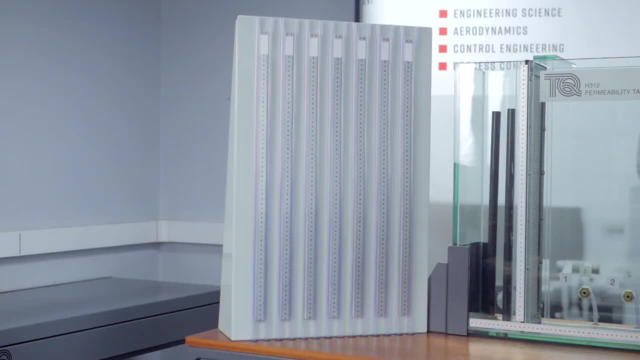 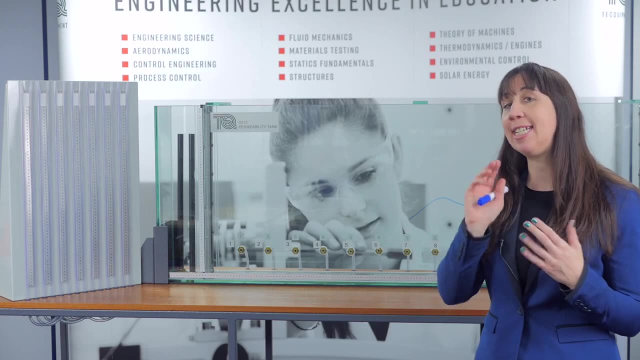 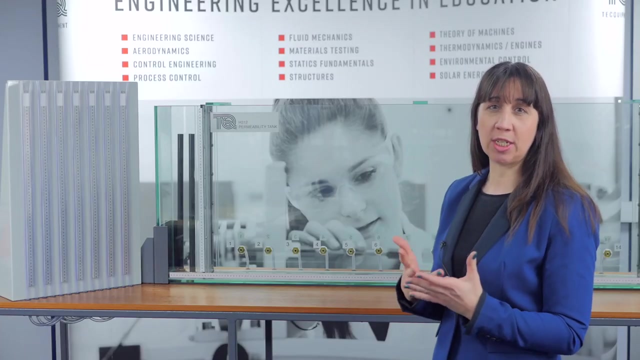 rate using the piezometer tappings along the side. This allows you to identify actual values of head along the flow path and demonstrate the distribution of head in seepage flow. The main part of the apparatus is self-contained and only needs a mains water supply and drain. 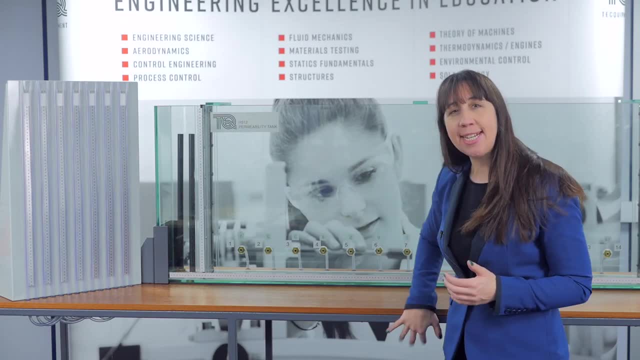 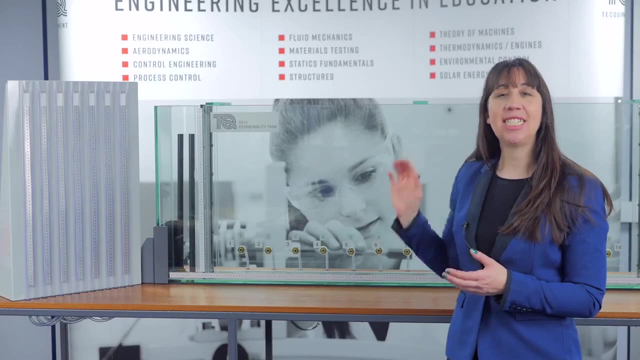 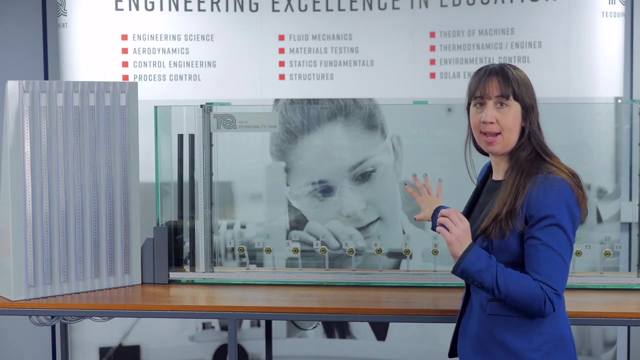 It consists of a transparent sided tank mounted on a sturdy steel frame bench with worktop that measures almost 2.5 metres in length, 1.5 metres high and 700 millimetres in depth. The clear plate glass on the side gives you full visibility of flow patterns and has a 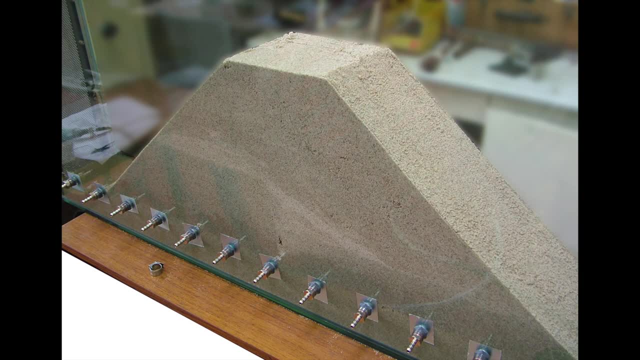 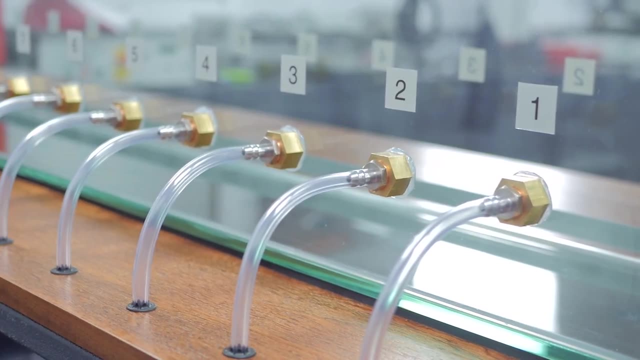 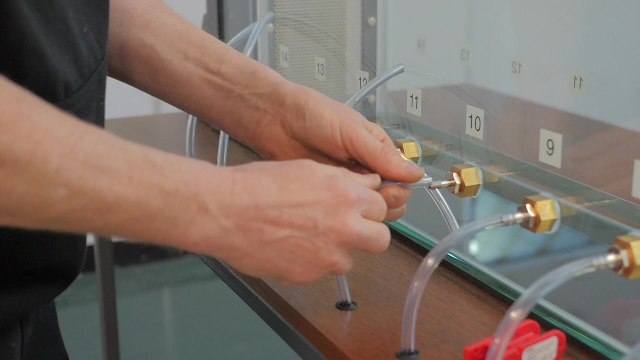 composition that resists abrasion from sand or the other permeable medium used Round the back. here you can see fourteen pressure tappings, each with their own filter for the water, for preventing unwanted particles getting into the working area. These tappings connect to a bank of piezometer tubes at the side of the apparatus, which allow 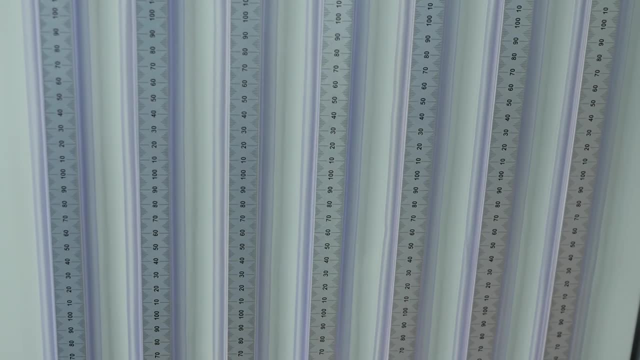 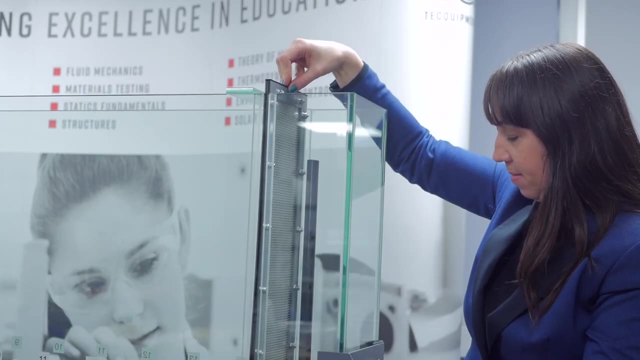 you to measure the head distribution along the tank. Removable stainless steel mesh baffles at each end of the tank hold the sand in place. At each side of the baffles are end compartments with adjustable flow pipes for setting the water levels at each end of the model. 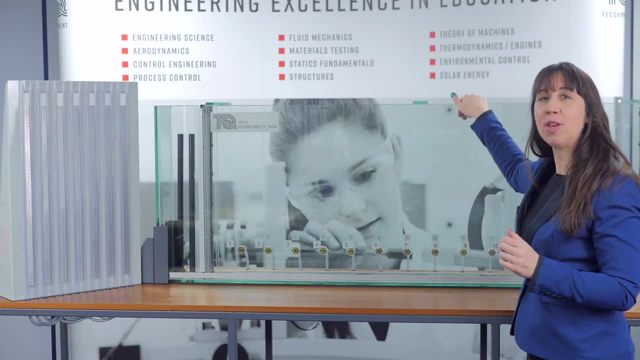 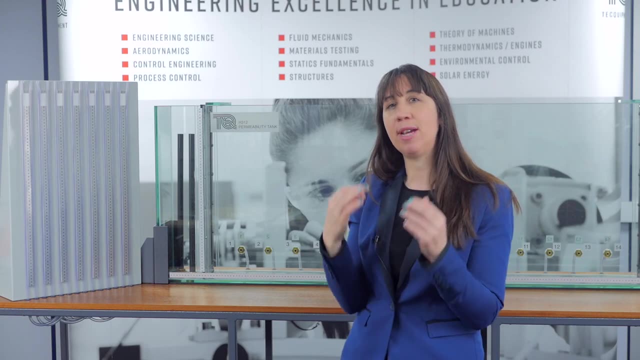 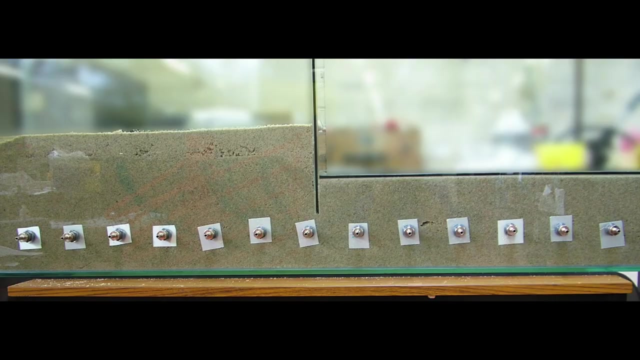 Let's look at the top now, which is open, so allow you to easily fill the tank and set up model structures. With the models, students are looking to replicate scenarios where water is retained behind a solid structure, standing on a permeable stratum, and identify the water exerting an upward 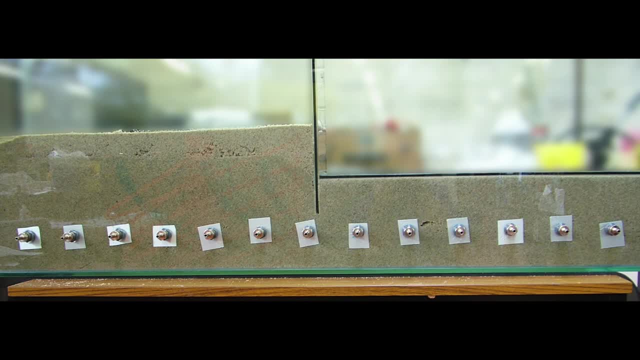 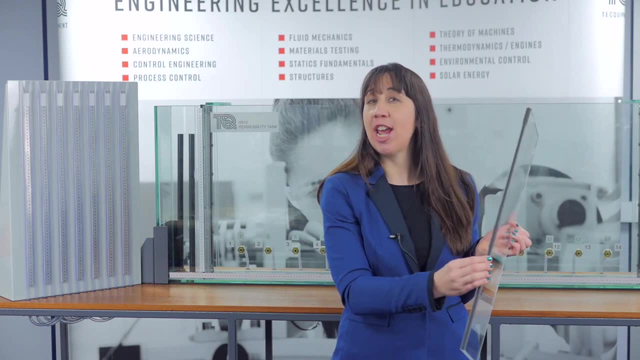 force or upward thrust on the base of the structure. We supply the material for making the models, which come in the form of clear, self-sealing sheet piling for creating walls and simulated dams. You might also notice these signs. You might also notice these signs.